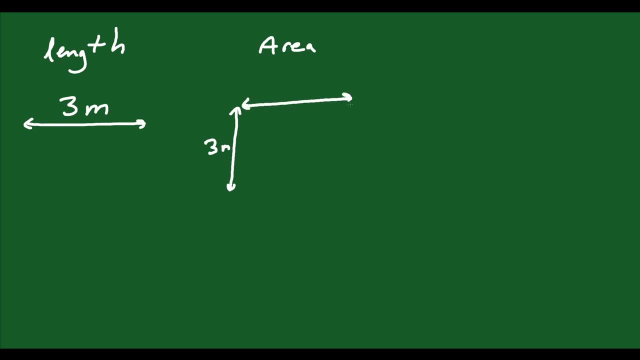 like three meters by three meters and this makes up a square. The area of this square would be three times three, which is nine meters squared The volume. if you want to talk about volume now, you can make a cube just like this, so a three-dimensional shape. So if you want to, 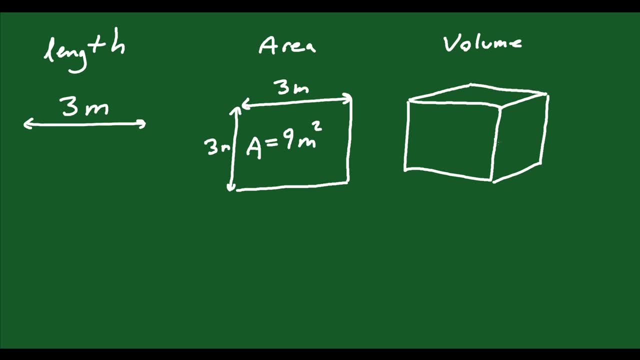 think about volume. you can think of it like this: Like this is a container and you're filling it up with water, right? How much water would fit into this container? So each of these sides, we could say, is 3 meters. still, right? 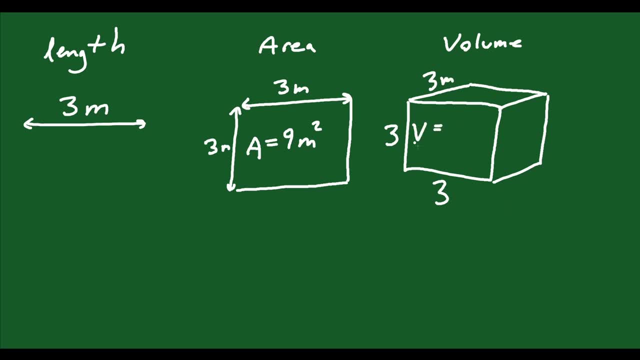 It's all in meters. The volume would be 3 times 3 times 3, which is 27 meters cubed right. So we can think about this in another way. When we talk about length, we can say that's 3 to the exponent 1,. 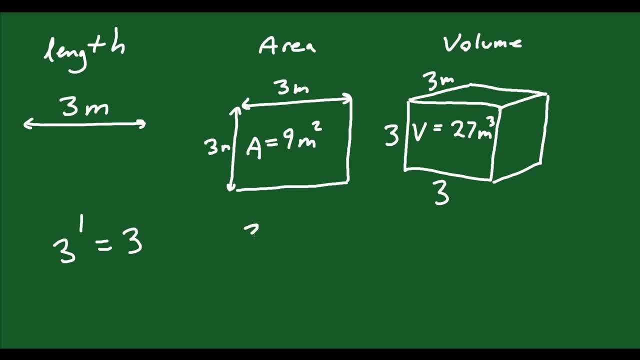 because that's equal to 3.. When we're talking about area, you can say that's 3 squared, because that's equal to 9.. You get your 9.. When you talk about volume, you'd say 3 cubed. 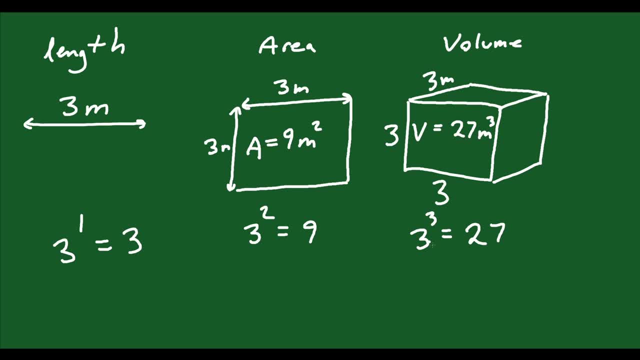 Well, that's 27,. right, You get your 27.. So that's one situation. right, when we have a length of 3 meters. But what if we have a length of something else? What if we have a length of 4 meters? right, 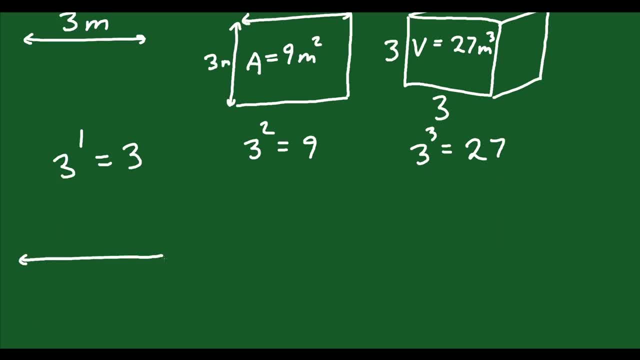 So let me scroll down here a little bit. What if my length is 4 meters? Well then I'd have 4 to the 1,, which is, you know, 4, same as we did here, If you have a square. 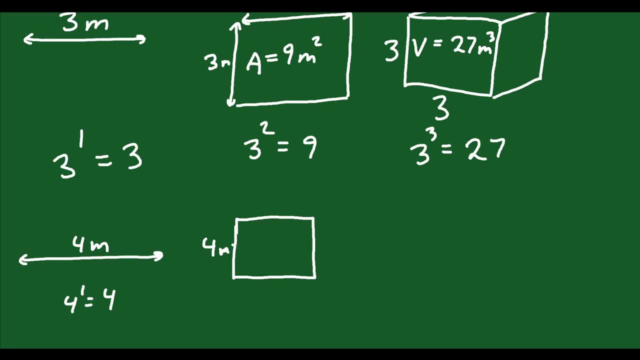 which is 4 meters by 4 meters. then you have: what is it? Well, it's 4 squared, which is 16, right? So this is going to be 16 meters. squared is your area. When we talk about volume, you draw your cube, right? 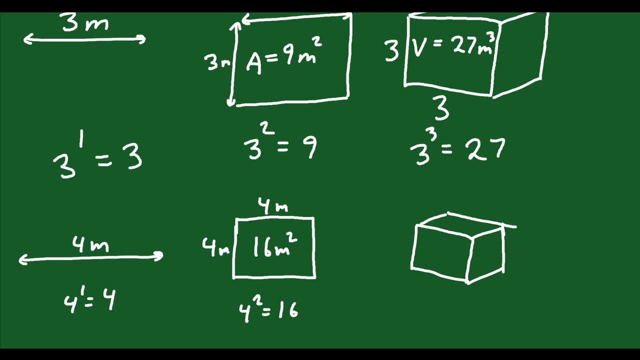 Something like that. They're kind of tricky to draw. That's okay. You have 4 by 4 by 4.. That's 4 cubed. That's going to be 64 meters cubed, right, 64.. 64 meters cubed. 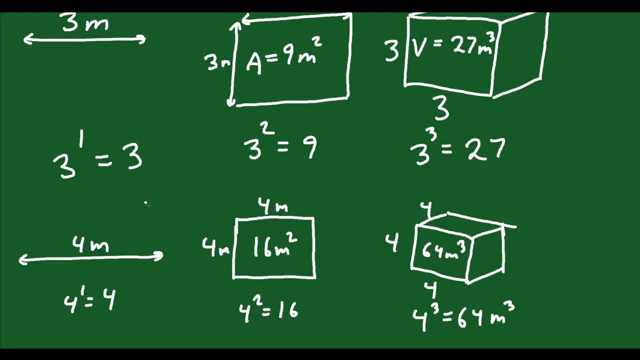 What do we notice? Well, for the length you went from 3 to 4, right, 3 to 4 is an increase of 33%. Okay, So you went from 3 to 4.. The difference there is 1..